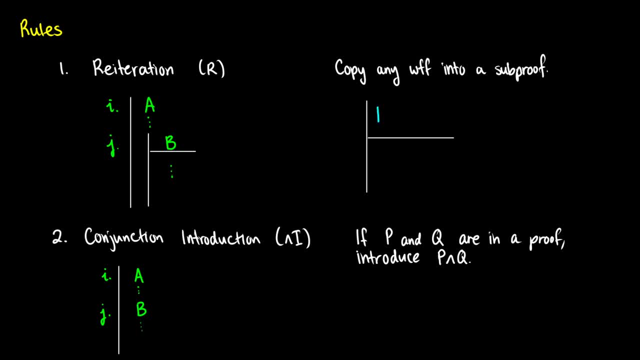 we have a line and what we do is we put our hypotheses above that line and all of our inferences occur after it. Now you can add more hypotheses at any point, as long as a rule is being used, and we'll talk about those rules by starting a new proof inside. 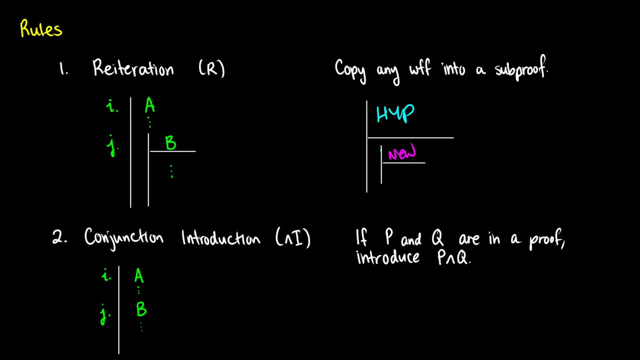 So you can add in a new hypothesis that has to eventually conclude. If you have, let's say, some hypothesis a or some line earlier in the proof and you have a new sub-proof b, so you're introducing like an extra step. 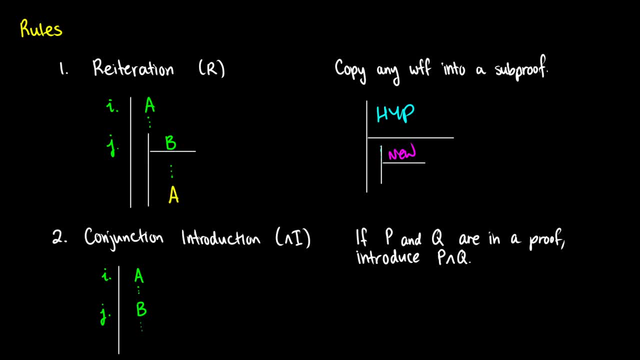 at any point. what we can do is we can reintroduce something from outside the proof. So let's say, in line k, later we can take it from line i and we can reiterate it with r. Now, in some systems you just assume that everything's already there, but reiteration is a way of explicit. 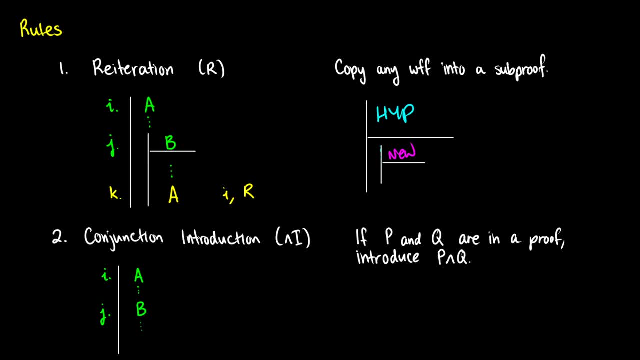 introducing it again. It's sort of like in our truth trees when we had branching paths and we introduced that variable in again. just to make it explicit. Okay, so we'll see reiteration in action a little bit later. Basically that means that if you have 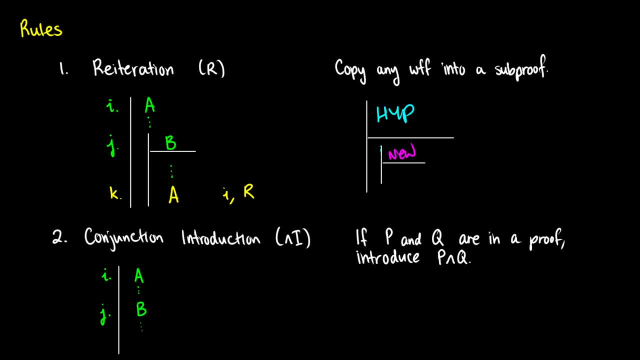 something earlier in the proof you can just copy it again. Conjunction introduction is nice. So if we have two lines, i and j, where you have say a in line i and b in line j, then later, let's say in line k, we can introduce a and b. So what we do is we write which lines we get it from. 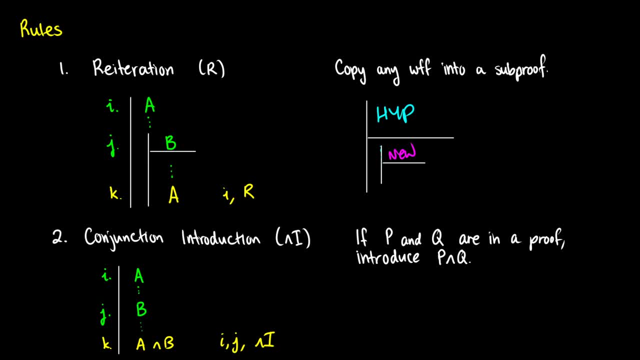 we got it from i and j and this is what's called AND introduction or conjunction introduction. So basically it says if you have p and q in a proof, you can introduce p and q. So to show this more explicitly with this example, suppose we have two hypotheses that 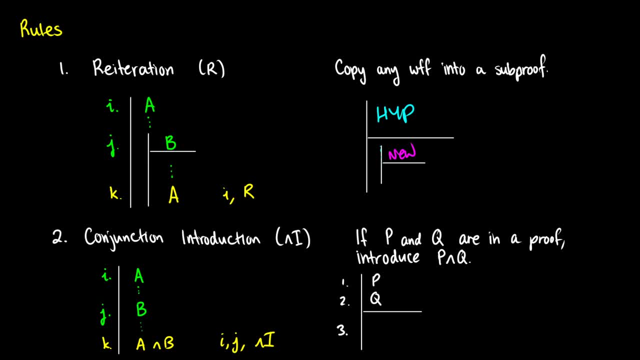 we're starting out line 1 and line 2.. We have p, we have q. then in line 3 we can introduce p and q, Line 1,, line 2, and and introduction. So this makes sense from a truth table. 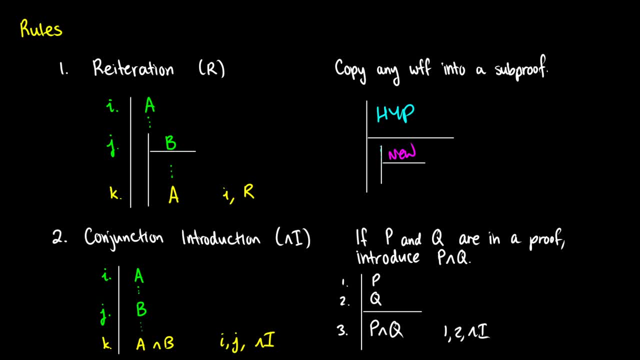 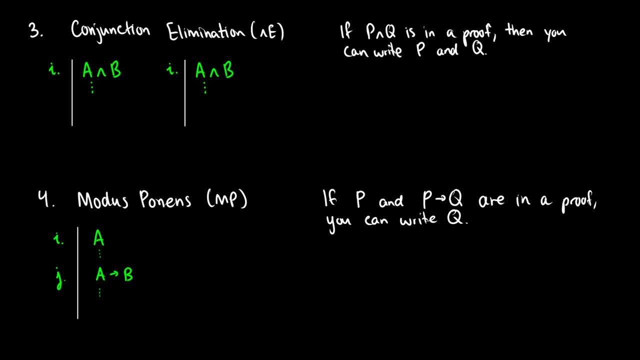 P is true, Q is true. therefore, P and Q is true. The third rule we have is called conjunction elimination. So basically, if A and B is true, we know that both A is true and B is true. So there's two different ways you can use the rule. 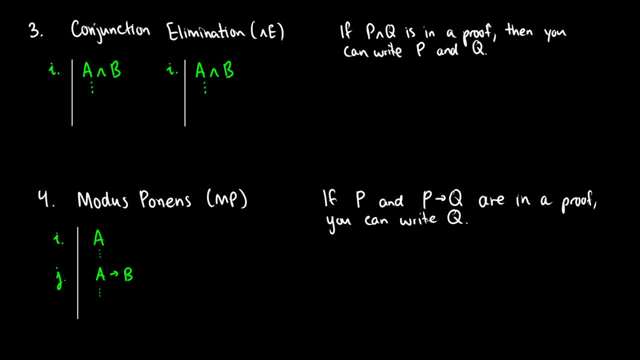 Either I'll do this in yellow to make sure that we're seeing the rule in action. So either you can put A down and you would justify this by saying: oh, line I, this was, and elimination or conjunction elimination, Or we could take B and this would also be from line I, and this is conjunction elimination. 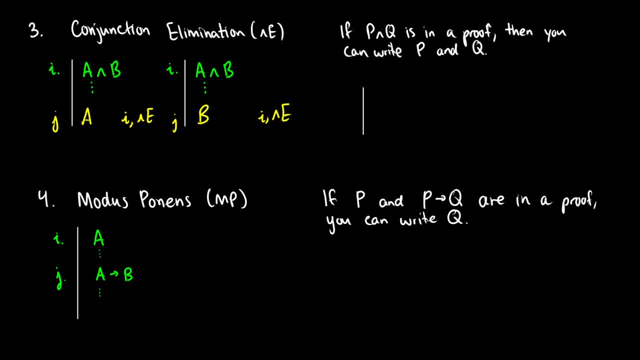 So specifically, if we want to see the example with P and Q, let's assume that we have P and Q somewhere in our proof. Let's just say it's the hypothesis, for instance. Then right away Let's say in line 2, and in line 3, say we could put P in line 2, and we could put Q in line 3.. 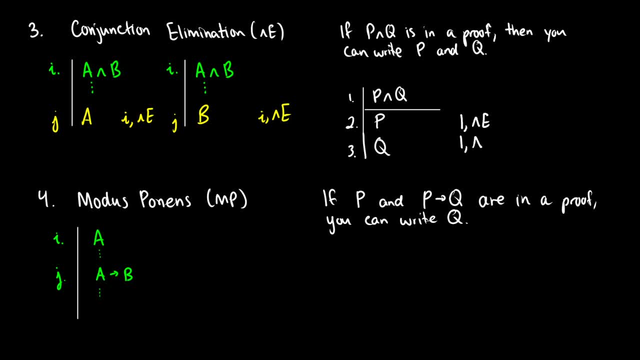 And both of these would say, oh, it comes from 1, it's and elimination. Okay, and then later we could put them back together if we want to. So that's conjunction elimination and conjunction introduction- Probably the most intuitive rules out of literally everything. 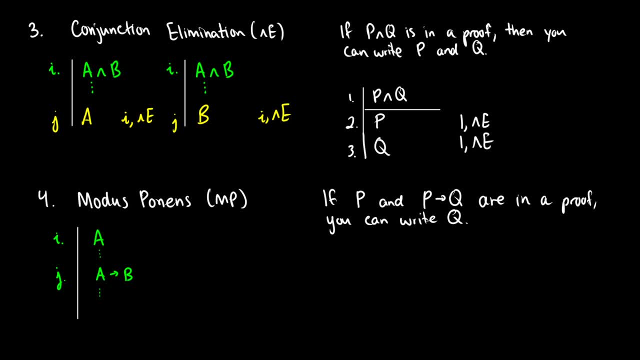 Now the one we saw in the very first slide was called modus ponens. Some people call this conjunction Conditional elimination. I like modus ponens, it's just how I learned it, And we abbreviate that as MP. So basically, if we have A and we have A arrow B, we can just follow the arrow. 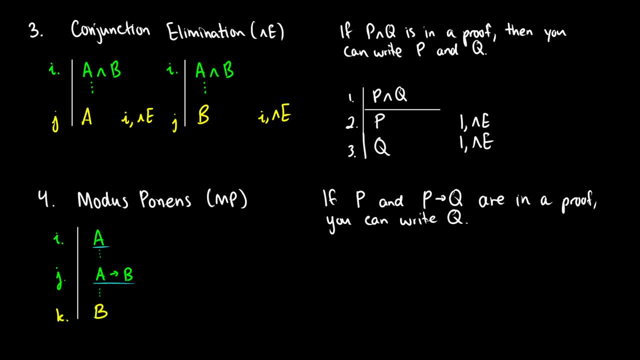 So in line K we can write down B. So you can justify this by saying: from line I and line J we used modus ponens. So basically we just follow the arrow and get the consequent Antecedent, then consequent. we had the antecedent, therefore we get the consequent. 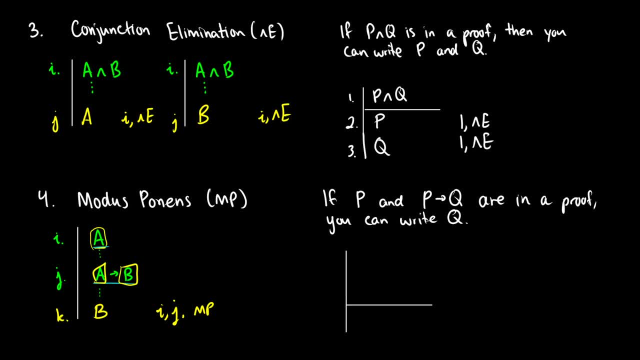 So this looks just like it did on our first line. Let's say we have P, arrow Q, let's put that first, why not? And then we get P In our third line. we can get Q by saying: from line I and line II we have modus ponens. 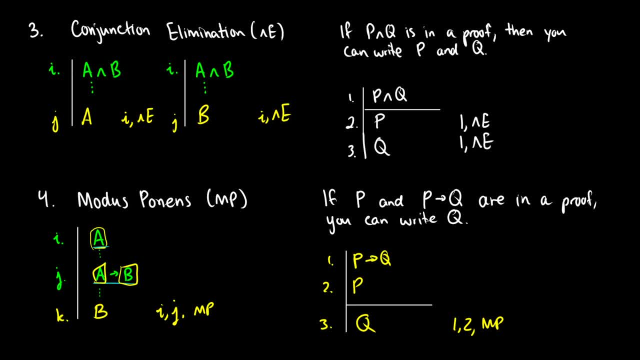 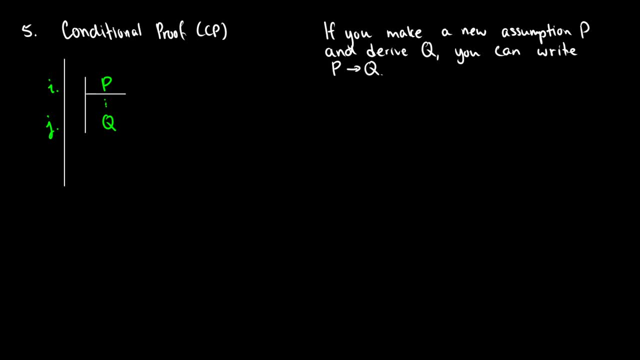 It doesn't matter the order of the 1s and the 2s. As long as we see those two patterns, no matter what order they're in, we're good. Okay, that's modus ponens. The last one we have is something a little bit more complicated. 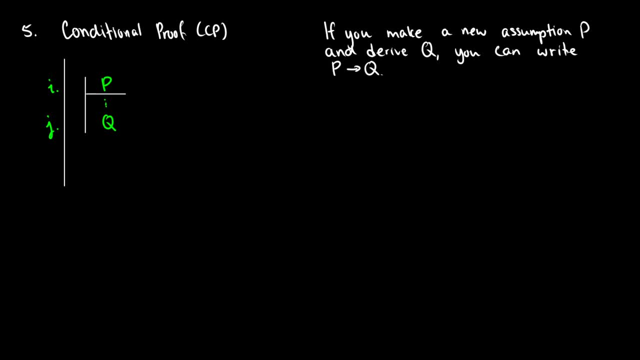 It's like the reverse of modus ponens. Well, not the reverse necessarily, but if you think of modus ponens as conditional elimination, you can think of this conditional proof as conditional introduction. So, basically, at any point we can start a new subproof. 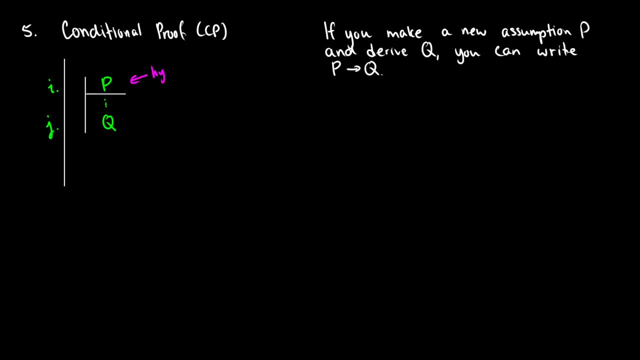 And if we add a new hypothesis, P, and we end up with a consequent Q, we've essentially said: okay, what if we have P? Well then we can get Q. So then in a, In a later line, in line K, you can write P arrow Q. 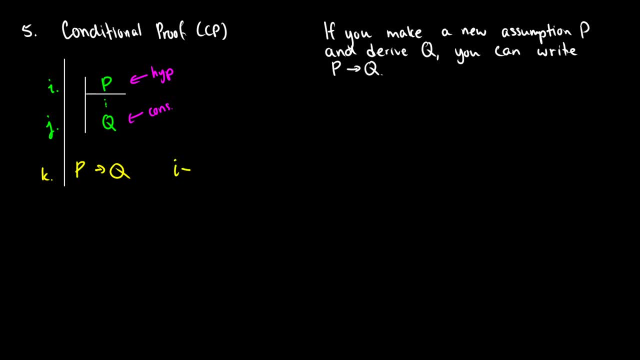 And what you do for this one is you justify it by saying, from line I to line J: we've proven P, arrow Q through conditional proof. So this is a hypothetical. This is what gives you that conditional. So this all has to be kept within the subproof though. 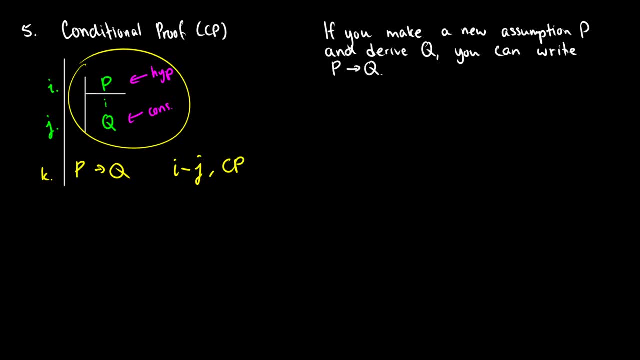 You cannot just take things from in the main proof and put it in there Like you have to do everything within the subproof And we'll see examples of that. So we just did that example before. But let's say, let's just make a new hypothetical example here on the right side. 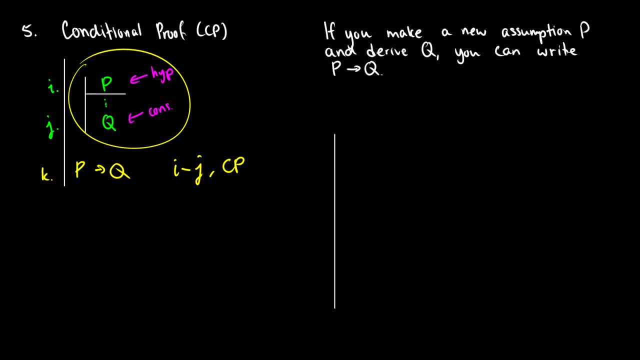 And let's do it with reiteration too. Okay, so let's say, in line 1, I start with C. This is my only assumption, So we'll call this the hypothesis, And what I want to do with this is: I want to prove that if we have A and B, 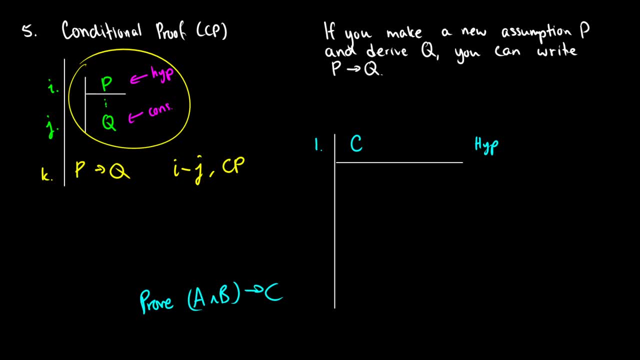 then we have C. That's what I want to prove. So what I can do is I can start a subproof. I can say: okay, well, hypothetically, hypothetically, what if we have A and B And we can add this as a hypothesis. 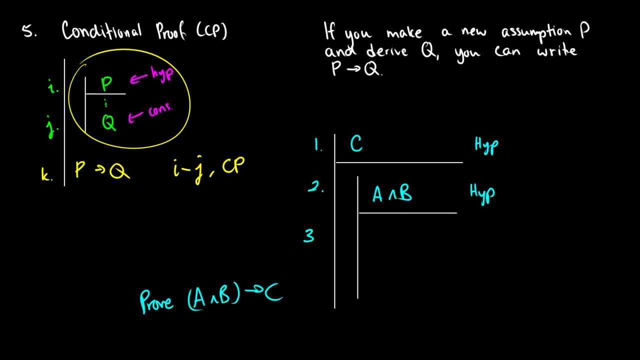 So what if we have that? Well, in line 3, what we can do is we can say: oh well, we have C as a hypothesis already, So we can copy that into our subproof. So from line 1, we use reiteration. 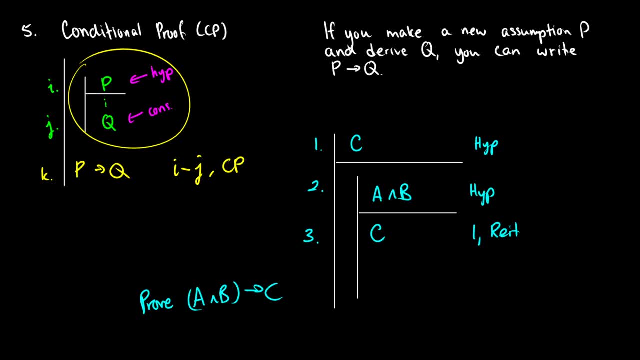 Okay, So from line 1, we use reiteration, I can write it R, I can write it REIT. Okay, Well, at this point we don't actually need our line to be this long, So let's just shorten that line a little bit to where it is. 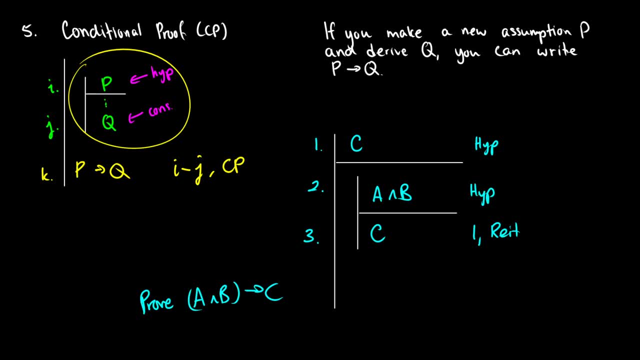 And what we've done now is we've proven that if we have A and B, then we get C. So in line 4, we can say, okay, A and B is our antecedent, And if we have that, we have C. 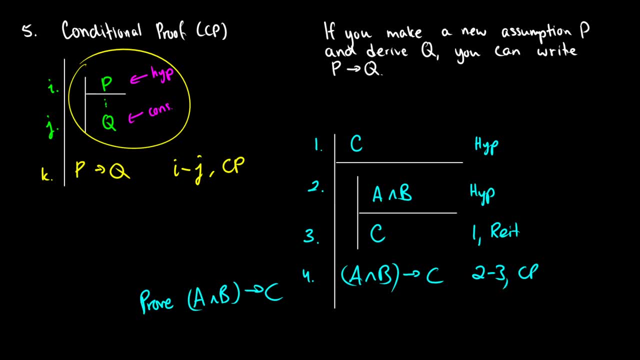 So from lines 2 to 3, we had a conditional proof. So that would be the end of our proof. We've shown that if we have A and B, then we have C, And this just follows naturally because we already assume that C is true at the very beginning. 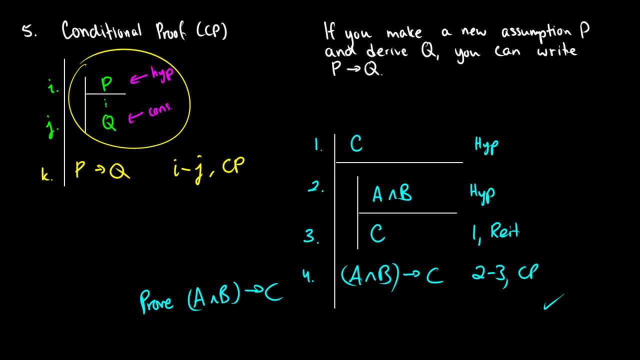 So actually what we could do here, just to really show you how powerful this proof is, you can take it from the very beginning, So you can consider the assumption from 1 from C as being a conditional proof. So in line 5, once we get rid of this little bar, we could say: okay, from C we get if A and B. 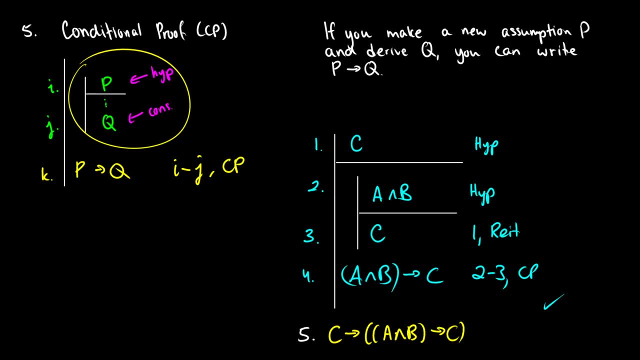 then we get C, And this is just a large conditional proof from 1 to 4.. So this is essentially the same thing: If we have C, then we have. if A and B, then C. So I like that example because it shows the conditional proof twice. 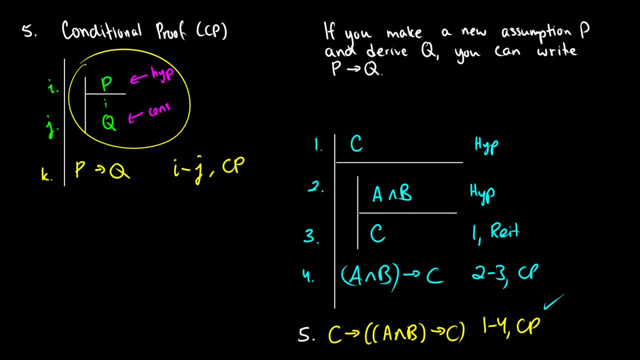 And actually it shows you what you're really doing in all your proofs. When you have hypotheses again, these are just like what-ifs. So almost every proof you do, theorem or non-theorem. in a way, it's just sort of a conditional proof. 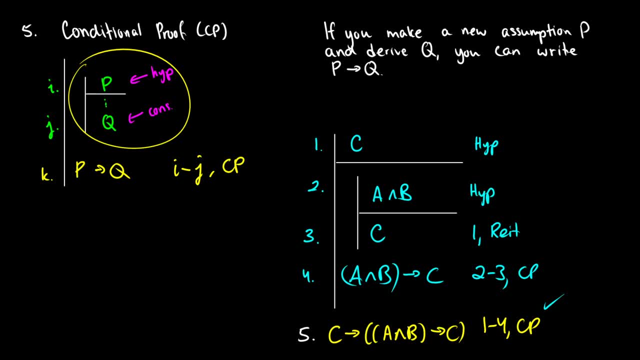 I shouldn't say that for every case. Tautologies are not conditional proofs, But if you have any sort of assumption and any sort of conclusion, you have a conditional proof. Okay. So let's do some examples. That's really the more important thing is just to show a bunch of examples. 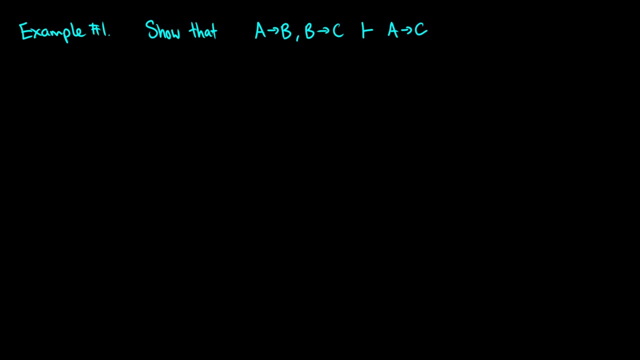 So I want to show that A arrow B and B- arrow C gives us A arrow C. So let's set up a couple rows here, Sort our assumptions one and two. Our assumption is that we have A arrow B And our assumption is A arrow C. 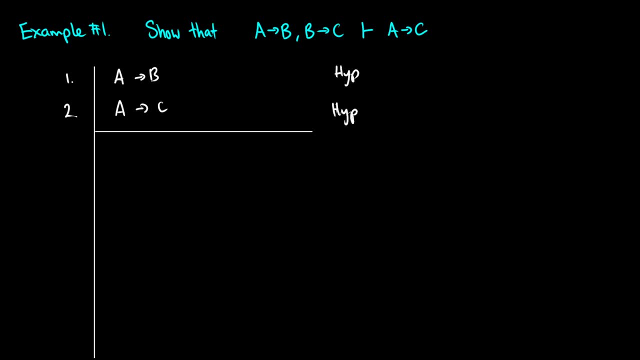 So this is our hypotheses. You never know how big these proofs are going to be, so just give yourself as much space as possible. Now we need to prove A arrow C, So what we should do is we know we're going to need some sort of conditional proof. 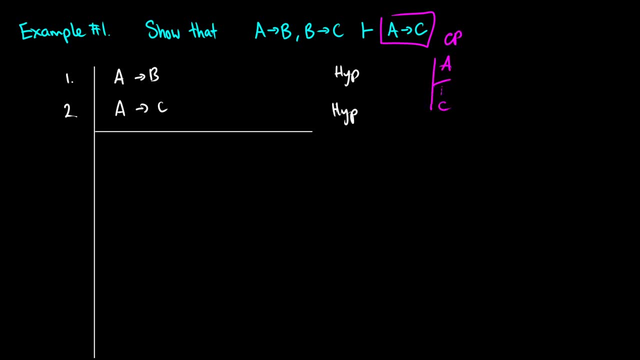 Because we have to assume A and we have to eventually get to C. That's how we get the arrow in our hypothesis And that's our final result. So in line three, I'm going to set that up. I'm going to start a subproof. 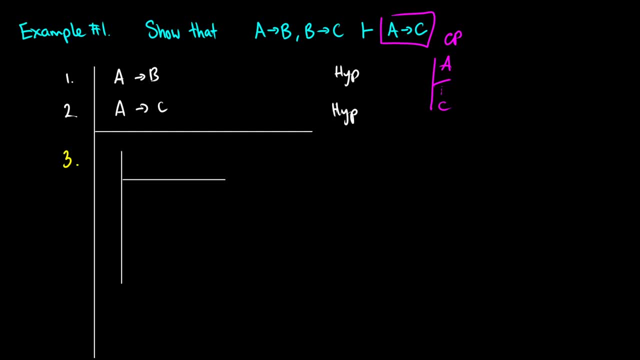 I don't know how long that's going to be, Let's just say it starts here. If I need a longer line, I'll make the line longer And I'll assume A as a hypothesis. Okay, In line four. what can we do? 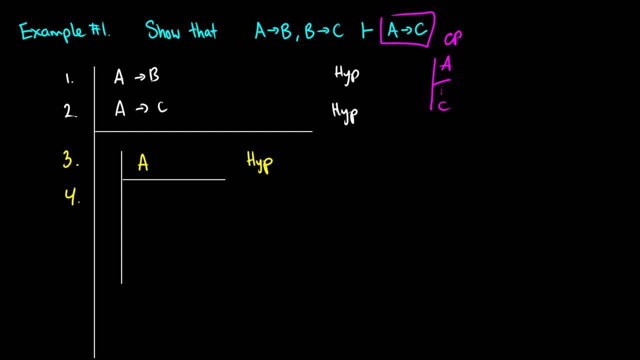 Well, I see that we have. Well, I should go back and fix my mistake here, Because we have actually that. this is B, Not A arrow C. So I see in line one that we have A arrow B, So I want to bring this back into the proof. 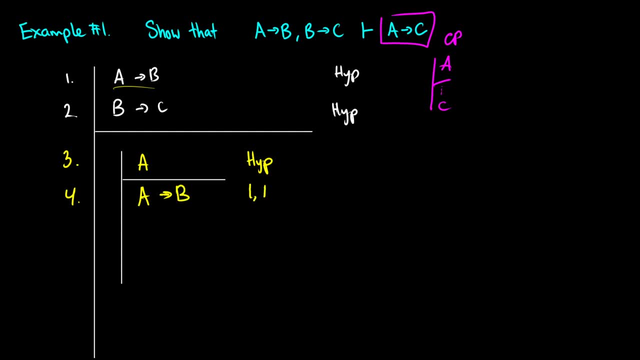 Because I can do something with it. So this comes from one and this is a reiteration Now in line five, because I have A and I have A arrow B, I have B. This is just an application of modus ponens from three and four. 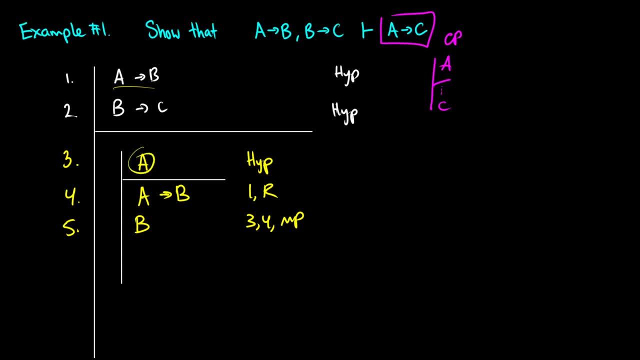 Or conditional elimination, Because I have A and I have A arrow B. therefore I have B And now I have a B here. Okay, Well, in line six I can reiterate B arrow C, Because I can do something with that. then 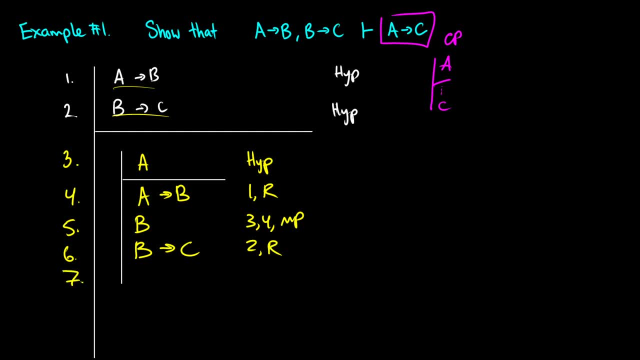 So from two, I'm reiterating it. And then in line seven I can take B, I can take B arrow C And I can apply modus ponens once again to get C out. So this is from five and six. 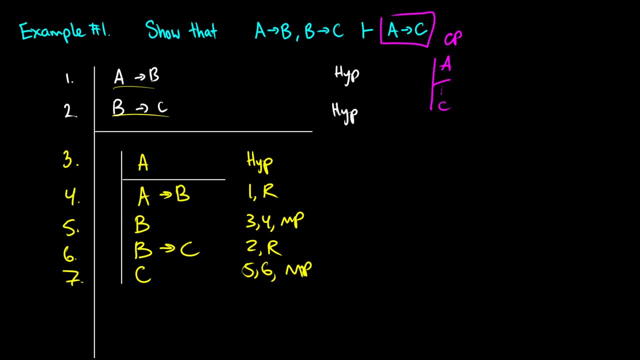 And this is modus ponens. So at this point I've started with A And I've proven C within that sub-proof. Therefore, in line eight, what I can do is I can introduce A arrow C using the conditional proof rule. from lines three to line seven. 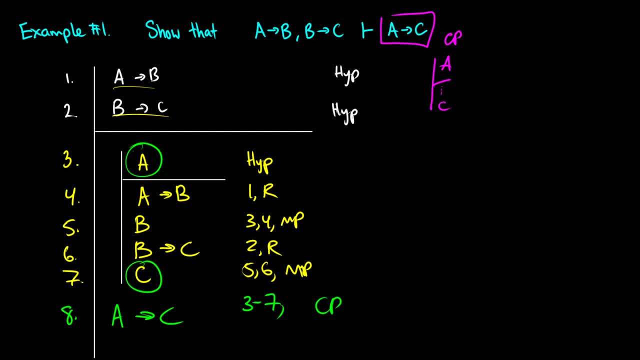 So I said: well, what if I have A And I've shown that with the assumptions I have, I can get C. Therefore, from three to seven, if I have A, then I get C. That gives us A arrow C. 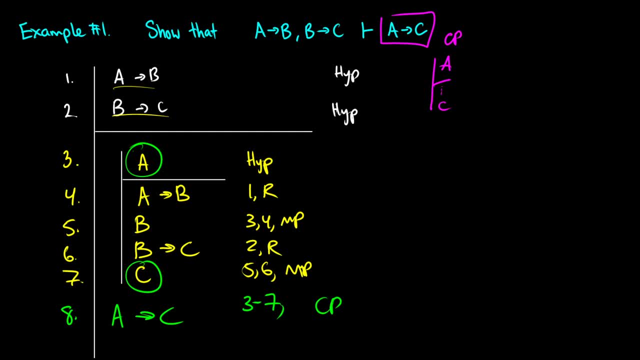 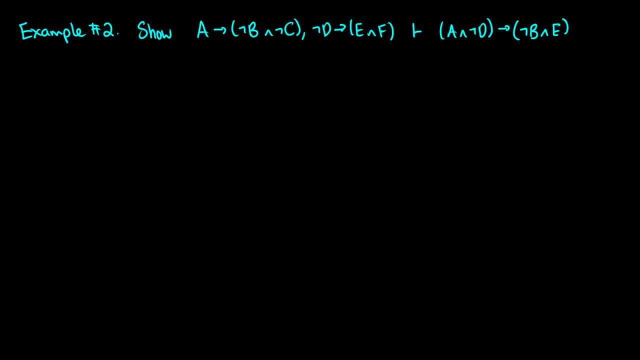 So that was the proof of example one. If A then B, If B then C. Therefore we have: if A then C. Let's do another example. This one's a little bit more. So if we have A, then we have not B and not C. 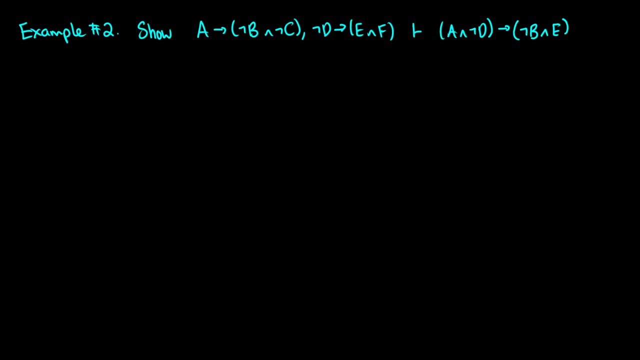 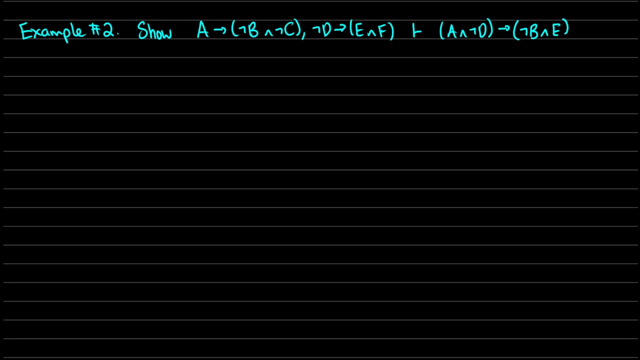 If we have D, then we have E and F. Therefore, if we have A and not D, we should get not B and E. I'm going to turn on the lines for this one because I have a feeling that this one might be a little bit long. 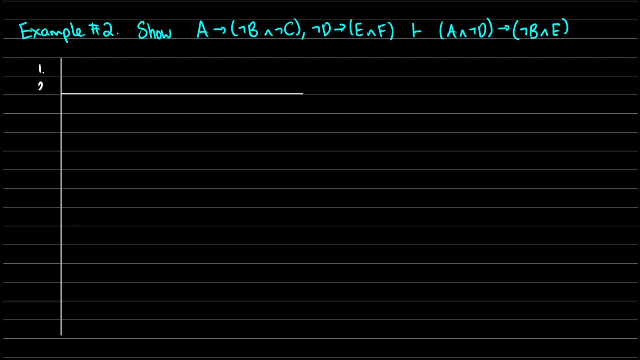 So I have two assumptions here. I'll turn the lines off at the end so that way we can see it in all of its beautiful glory. So if we have A, then we have not B and not C. That's our first assumption. 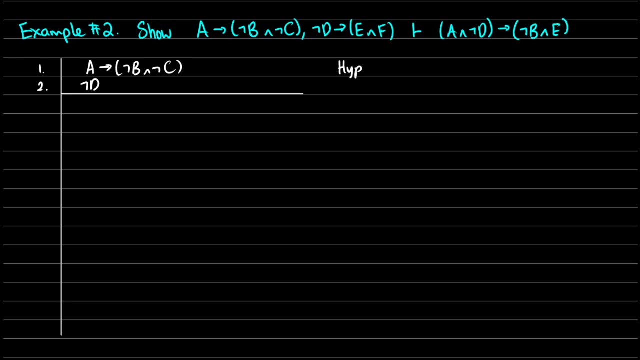 Our second assumption is that if we have not D, then we have E and F, And we want to show that if we have A and not D, we get not B and E. So because I see an arrow here, I'm probably going to have to assume: 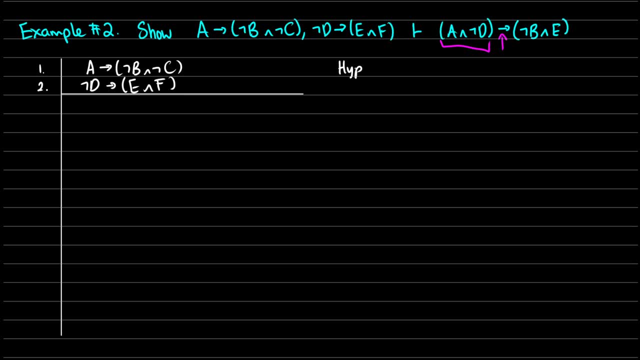 that we just have A and not D And then see what happens. So let's set that up. I don't know how long it's going to have to be, but we can put some lines in here. So for my assumption, I'm going to say: 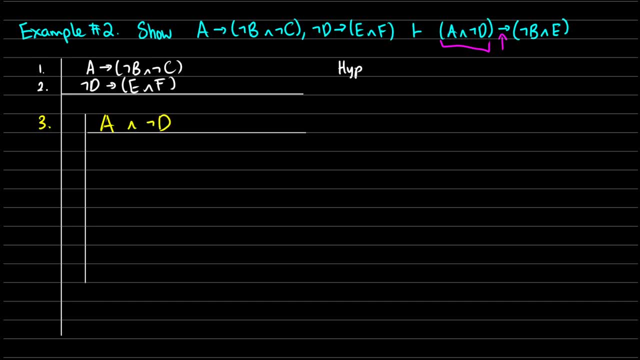 okay, what happens if I have A and not D? So this is another hypothesis. Okay, well, here we can use conjunction elimination. So 4 and 5, we're going to get A, we're going to get not D, And this is just conjunction elimination. 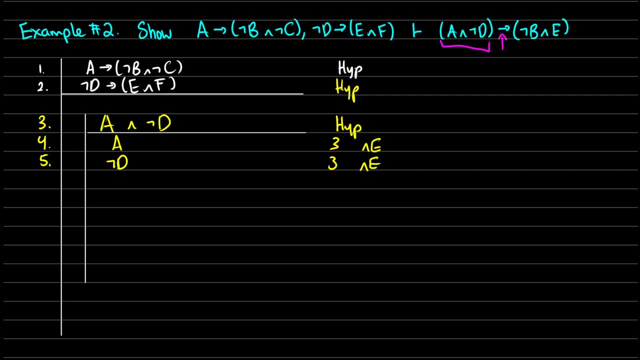 On 3.. Okay, Well, at this point I have A, I have not D, And in 1 and 2, I see some modus ponens potential. So in 6 and 7, I'm going to reiterate these rules. 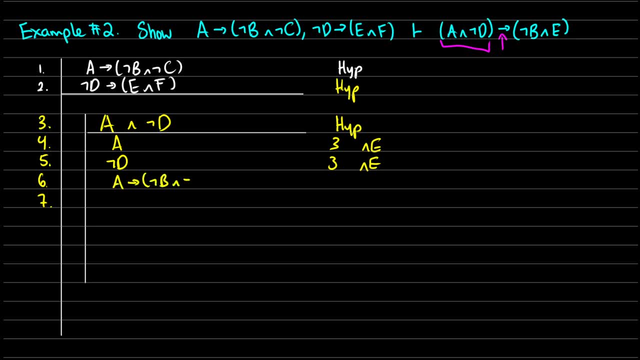 so that way we can use them in the sub-proof. So if we have A, then we have not B and C. This comes from 1, that's reiteration. And then we're going to have not D arrow, E and F. 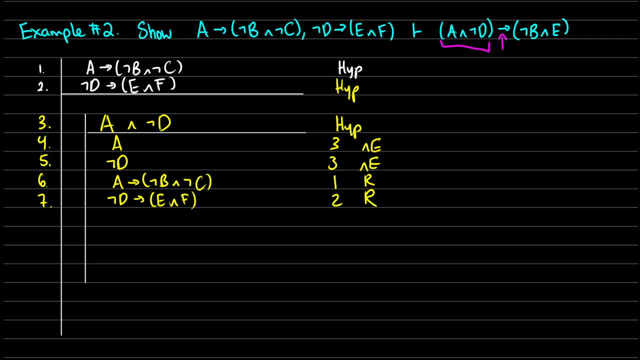 So this comes from line 2.. And this is reiteration. Okay, at this point we can use modus ponens. So in lines 8, we have A From line 4, we have A From line 6, we have A arrow, not B and not C. 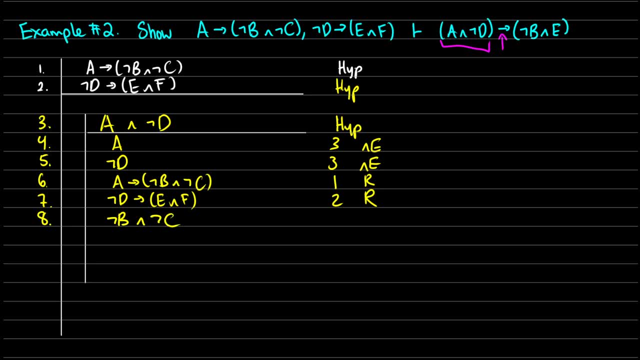 So we can use modus ponens to get ourselves not B and not C. So justification 4, 6, MP In line 9, we can do modus ponens again with not D and not D arrow, E and F. 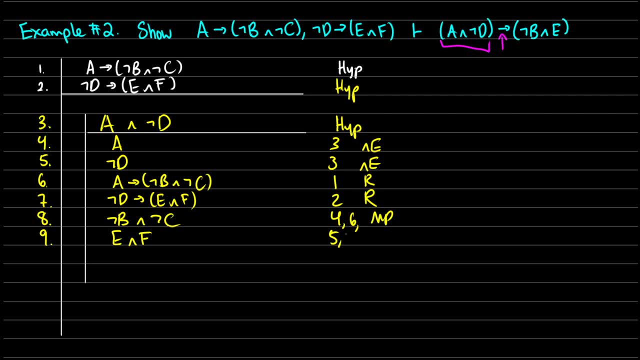 That gives us E and F. So this comes from line 5.. And line 7, that's modus ponens. So these two lines right here we get E and F. Now we have to remind ourselves: what do we want to prove? 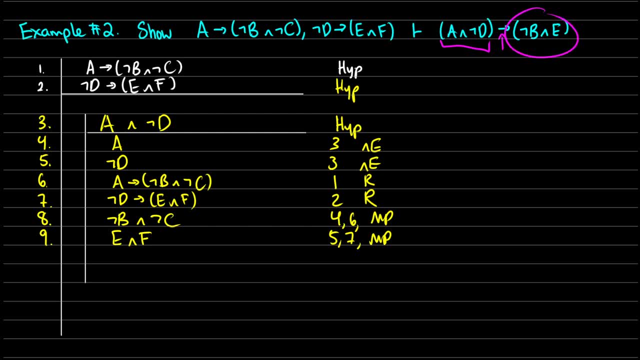 If we have A and D, we're trying to get that. we have not B and E. That is our goal. So I'm going to use conjunction elimination on 8 to get not B. So that's 8, and that's conjunction elimination. 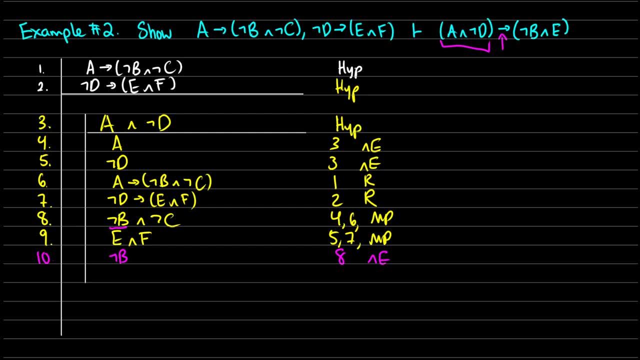 On line 9, I'm going to use conjunction elimination to get E. It comes from 9, that's another conjunction elimination. So now I have not B and I have E on their own. So I need to make this line a little bit longer. 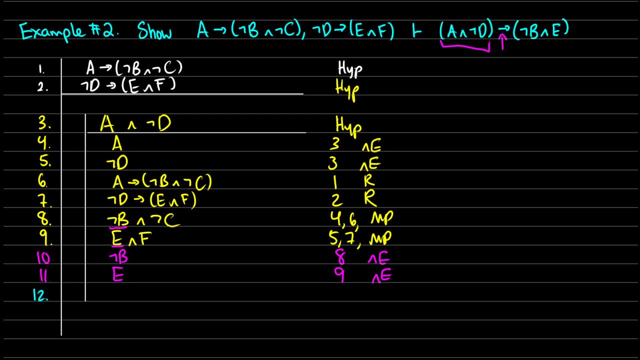 because I need one more line here. So on line 12, I'm going to take not B, I'm going to take E and I'm going to join them together Because we know those are both true individually, so they'll be true together. 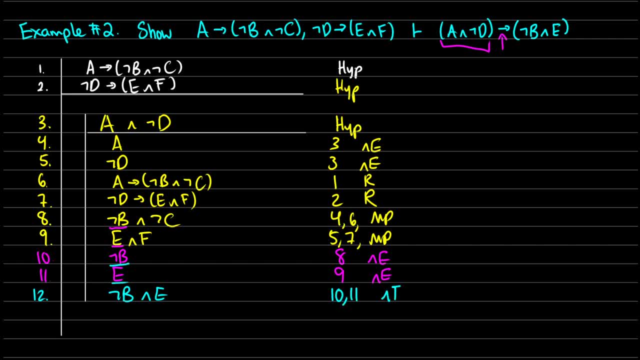 So from line 10 and line 11, that is and introduction. so now I have not B and E. So this concludes our conditional proof now, because we're saying if we have A and not D, then we're going to get not B and E. 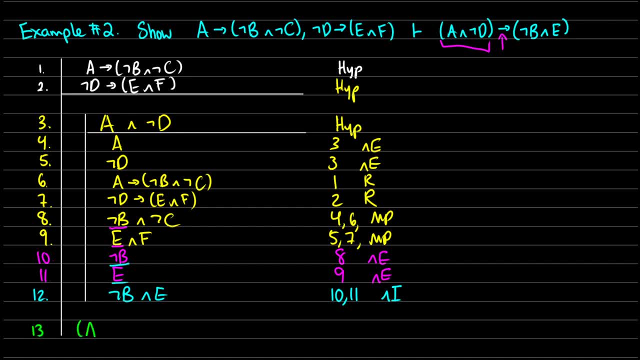 So for our final line in 13,, we can say, okay, if we have A and not D, then we're going to get not B and E. And what does this come from? Well, from line 3 all the way up to line 12,. 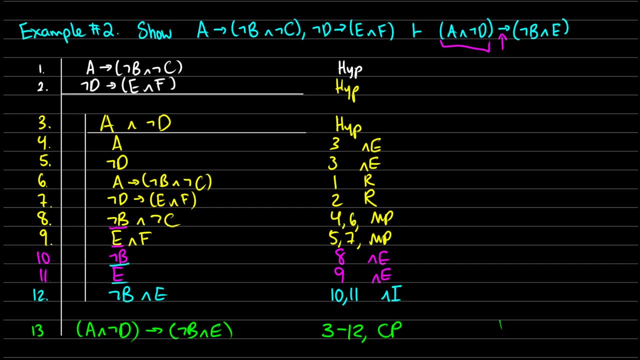 that was a conditional proof. And there we're done. We have shown that A arrow, not B and not C and not D. arrow E and F proves that if we have A and not D, then we get not B and E. Okay, so if we take out the lines, 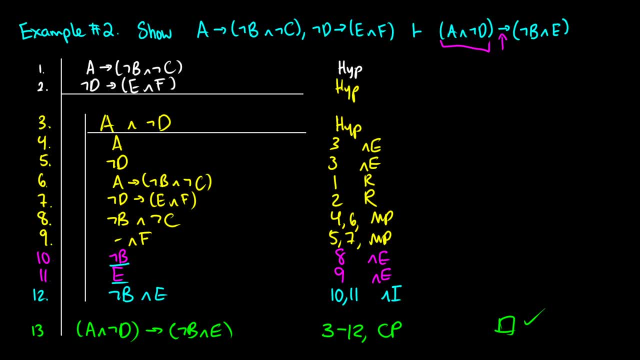 this is what our final proof looks like. We should get rid of these colorful lines, if we can. that way we can see what it looks like. Okay, So that was example number two, a little bit more complicated than example number one, but another good illustration of the conditional proof. 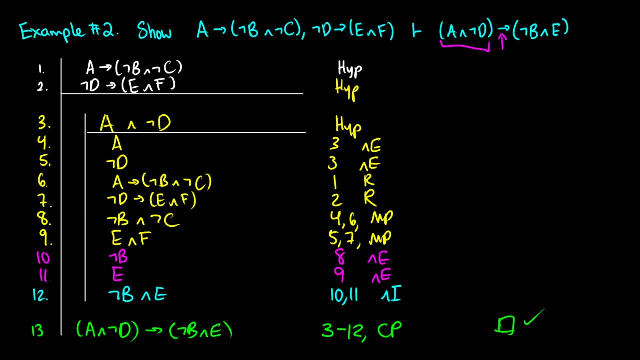 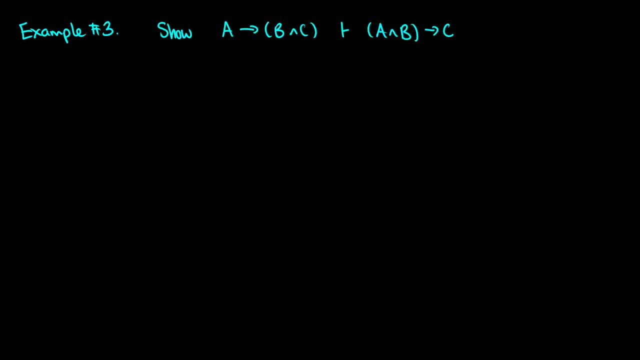 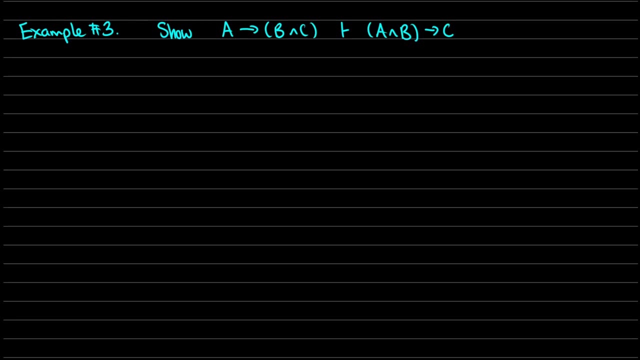 reiteration, modus ponens, conjunction elimination and conjunction introduction, Like everything we introduced was used in this proof. Now one more example: Show that A arrow B and C gives us. if we have A and B, then we have C. Okay, 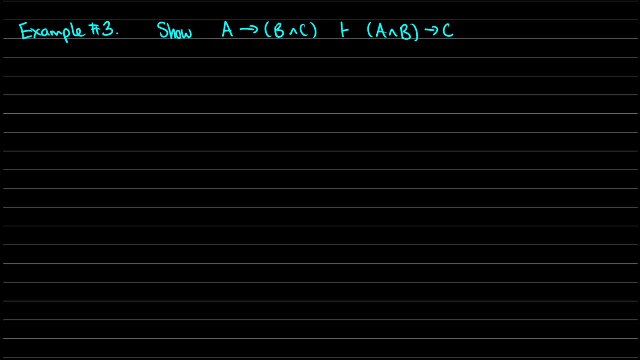 Here's an interesting one. It's interesting because you might think to approach it a little bit differently than how you should. So let's just set this up. Our only assumption we're given is that if we have A, then we have B and C. 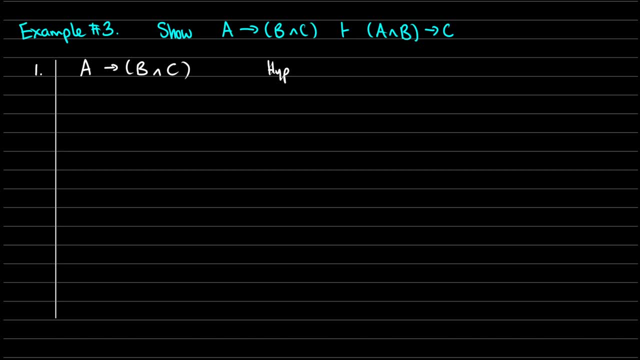 So that's our hypothesis, Okay, Well, we need to show that if we have A and B, then we have C. So what we have to do in the sub-proof is we have to make an assumption that we have A and B. 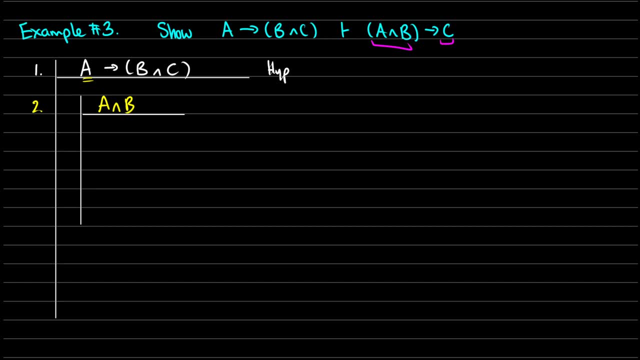 Now you might be thinking, hold on, we just have A here. why don't we just use A as an assumption? But no, you have to take everything on the antecedent as an assumption, otherwise the CP proof will not give us. if A and B, then C. 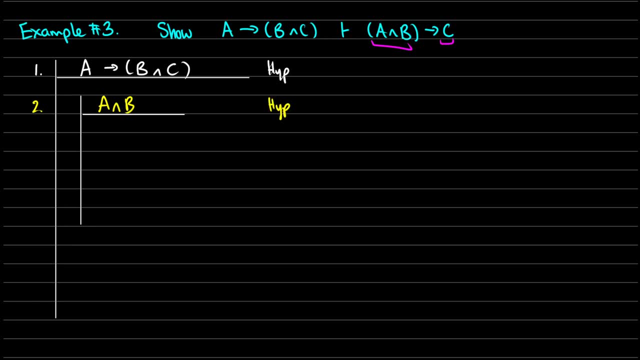 So that's a new hypothesis In three and four. what we're going to do is we're going to use conjunctions, conjunction elimination. Now, do we have to actually get B? We don't need B, So let's just use conjunction elimination to get A. 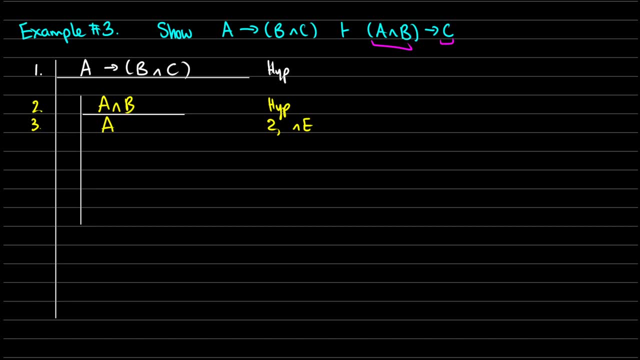 So two, conjunction, elimination. Why bother writing down B if we don't need to use B for modus ponens or anything? So we have A Four. we're going to reiterate our hypothesis: If we have A, then we have B and C. 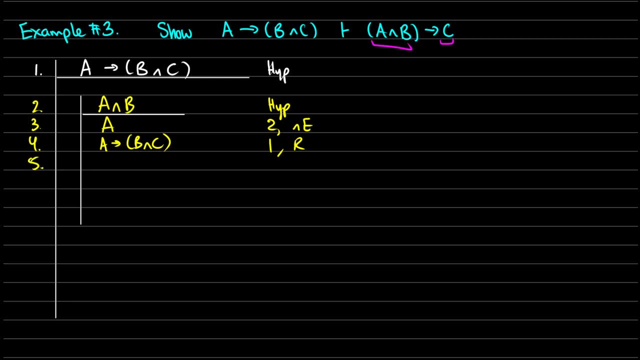 So that's a reiteration from one. In line five we're going to use modus ponens on A arrow, B and C to give us B and C. So from three and four we did modus ponens. Now at this point,